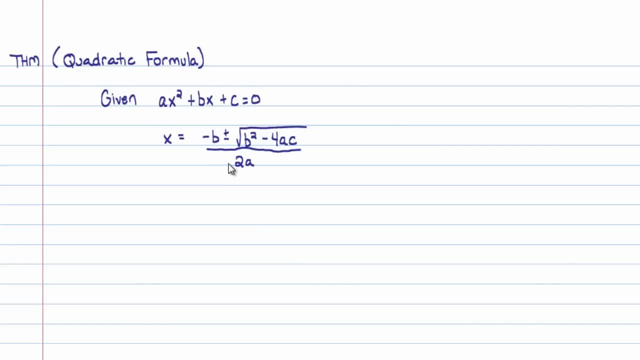 Before we go any further, I just want to remind you of the quadratic formula that we're given a quadratic equation of the form ax squared plus bx plus c is equal to zero. And given that quadratic equation, the solution is equal to negative b plus or minus the square root of b squared minus 4ac all over. 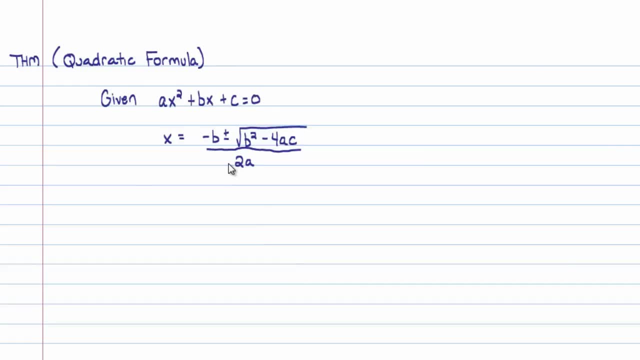 2a. And we're going to use that to solve a very specific kind of quadratic equation. 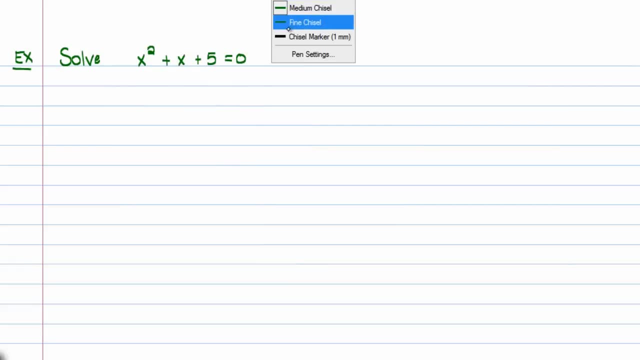 We'll go ahead and solve x squared plus x plus 5 is equal to zero. And as we've mentioned in previous video lectures, the first thing I'm going to try to do is factor this. So I'll take a look at this and see if it factors. x times x would give me the x squared. And the only way I can get two numbers that multiply to 5 is if this is 5. And this is 1. However, you could already see that this is not the way it's going to factor because this would give me a 6x for the middle term. So I already know this is not going to work. 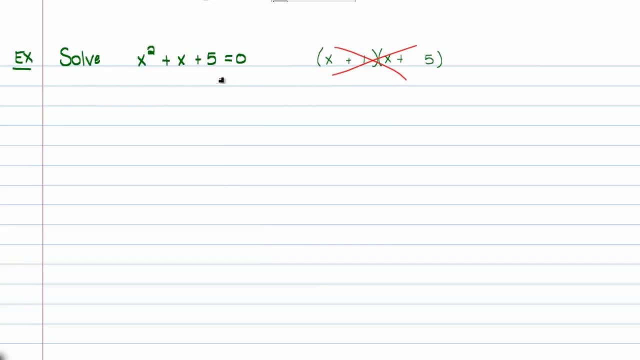 So it looks as though we're going to have to jump right into the quadratic formula here. The a for this is 1. So that's the coefficient of the x squared term. The b, which is the coefficient of the x term, is 1. And the c, which is the constant term, is 5. Using the quadratic formula, we get x is equal to the opposite of b plus or minus the square root of that b being squared minus 4ac all over twice the value of a. 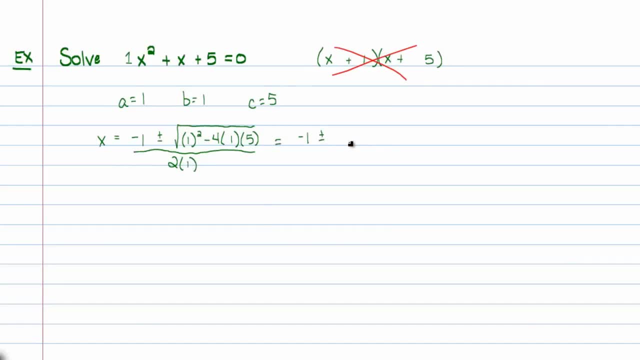 We'll go ahead and simplify this down. This is negative 1 plus or minus. That's the square root of. And you'll see that underneath the square root, I have 1 minus 20, or in other words, a negative 19. All over 2. 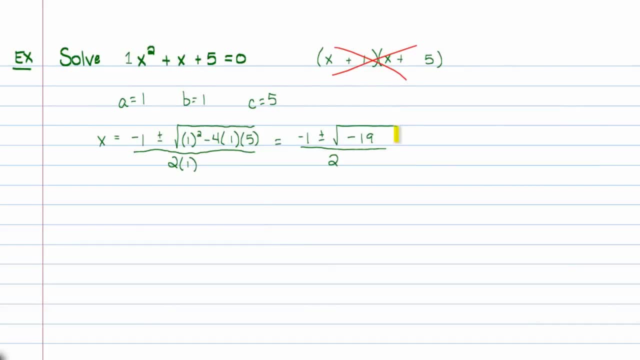 And this should be one of the first few rare moments where you have encountered a negative underneath the square root. Up to this point in mathematics, a lot of people say that have probably lied to you and told you that this number doesn't exist. 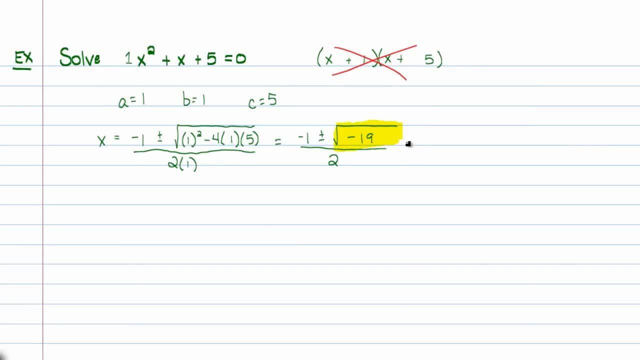 This number does exist, actually. This is just a special kind of number. Having a negative underneath the square root causes us to basically have to invent a new number system. Now, this number system that we're about to create was not formally defined until the mid-19th century. 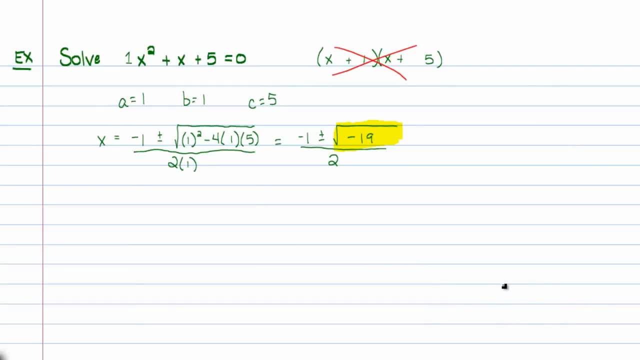 So it's a fairly recent addition to our mathematical set of objects. 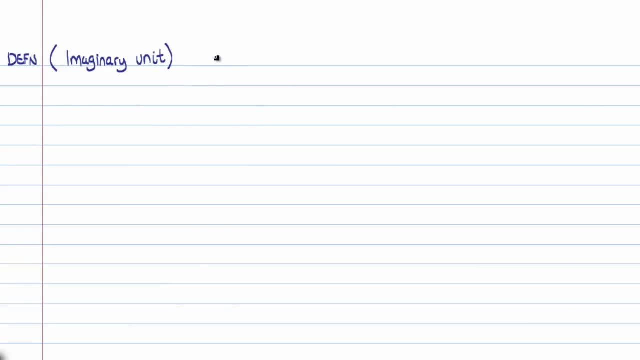 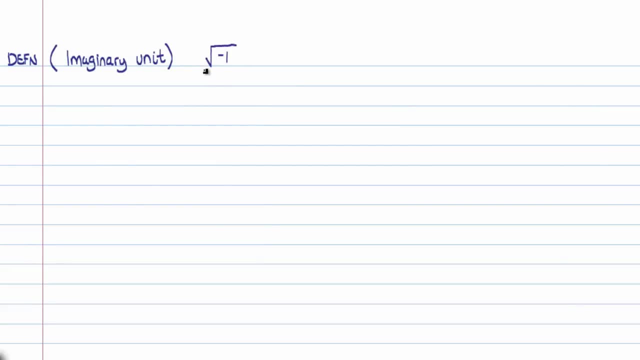 So the square root of a negative 1, the simplest square root involving a negative as the radicand, the square root of a negative 1 is defined to be i. So from this point forward, every time you see i, you should think, oh, that's the square root of a negative 1. 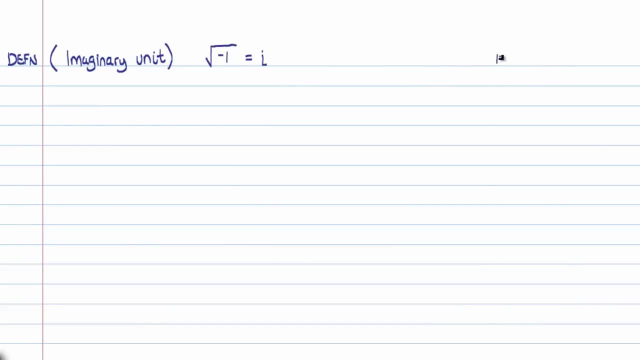 Just a symbol for it, just like pi is roughly equal to 3. 3.14 dot, dot, dot, dot, dot, okay? 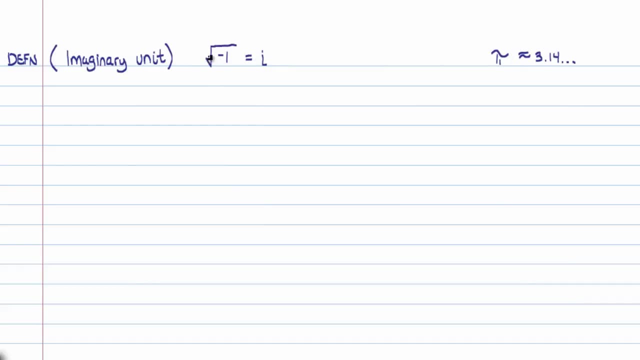 So it turns out that i is just our standard notation for the square root of a negative 1. 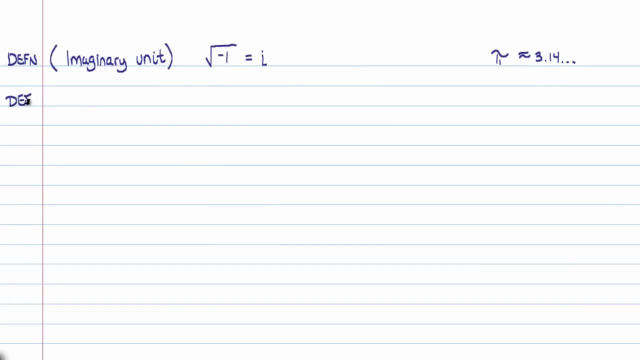 Well, this allows us to really introduce a whole new number system. 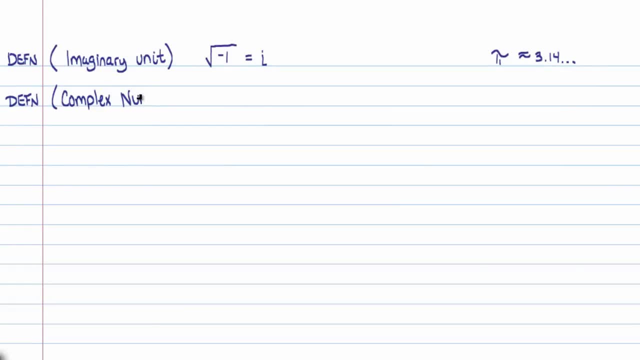 So I'm going to define first what a complex number is. A complex number is a number of the form a plus b times i, where a and b are real numbers. a and b are real numbers. And I just want to start introducing you to correct mathematical notation. 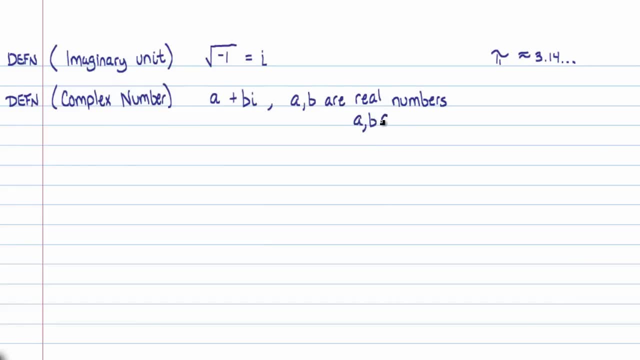 a and b are real numbers. A shorthand for that is this. a and b. 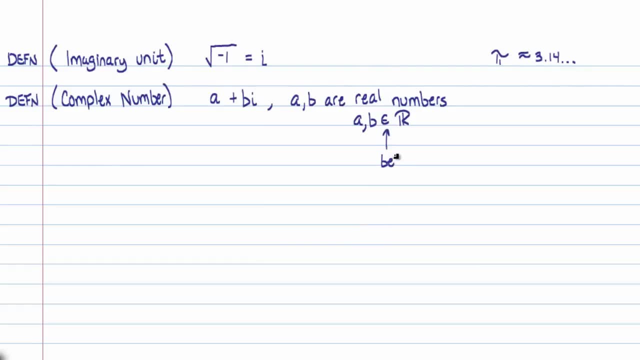 This means a and b. A belongs to, and that r right there stands for the real number system. Okay. So just to let you know, the a and b are real numbers. 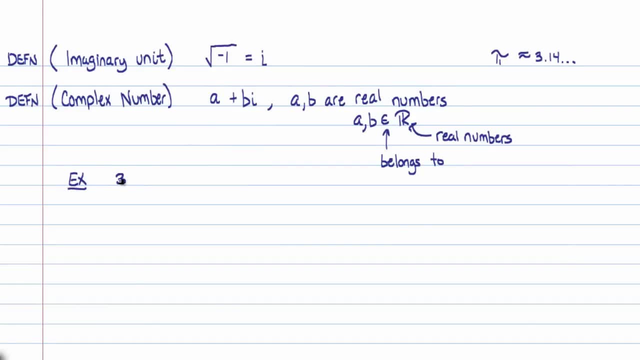 For example, some examples of complex numbers are like 3 plus 2i, or pi minus 1.1i. Or 3 sevenths minus 2 thirds times i. All of these are complex numbers. 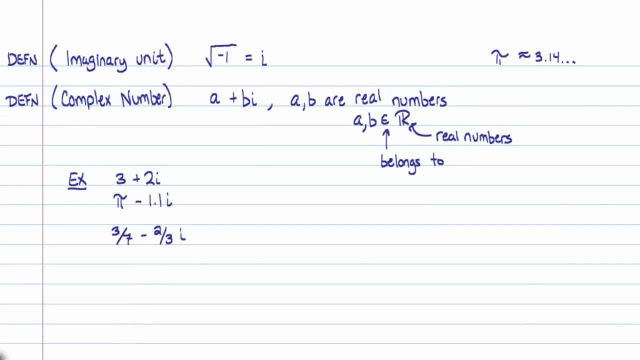 And in fact, it's a whole new number system. Remember, the number systems, if you view past through my previous lectures, we had these number systems, the natural numbers, the whole numbers, the integers, the rational numbers, the irrational numbers. All of those sets, specifically the rational numbers and the irrational numbers, when we combine them and grab them and put them in a container, we call that the set of real numbers. But this is a new set of numbers here, the complex number system. And it's just a set of all numbers of the form a plus bi. 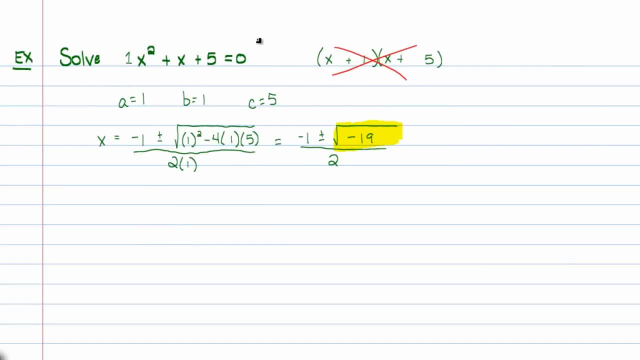 So going back to our example, how could I write this as a complex number? Remember, it has to be written as a plus b times i, where a and b are real numbers. 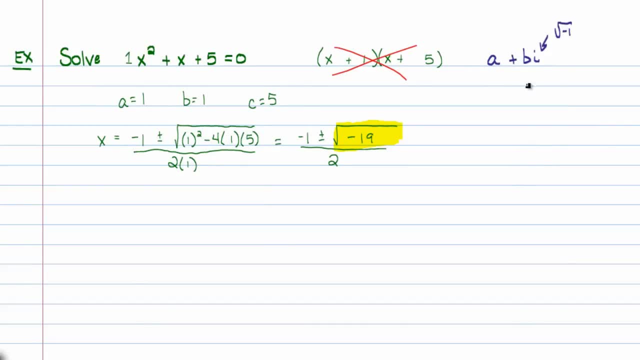 And i is just... It's just the square root of a negative 1. 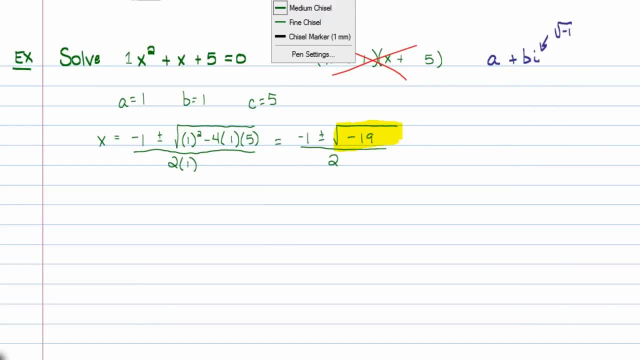 Well, here's how it's done. I'm going to switch my pen color here a little bit. And the first thing I'm going to do is break up this fraction. That fraction can be written as negative 1 half plus or minus the square root of a negative 19 over 2. 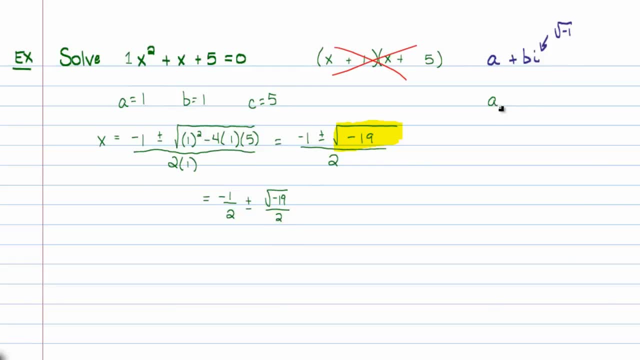 And this comes from a theorem you learned a long time ago. 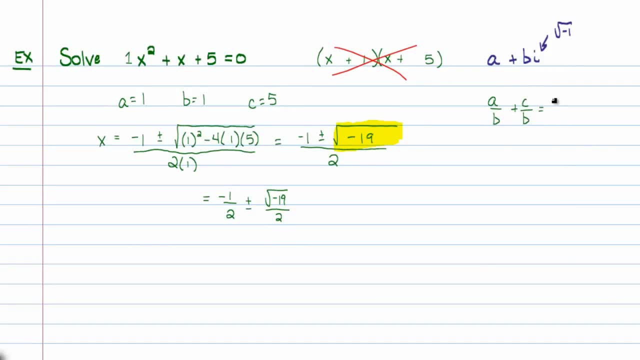 If you have a over b plus c over b, that's equal to... a plus c over b. 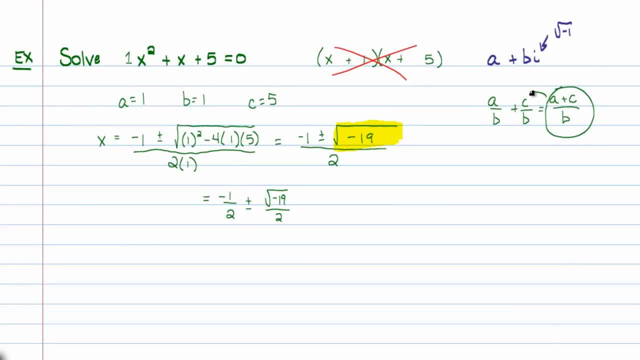 And all I did is I actually worked from this and split it apart. So it's a over b plus c over b. 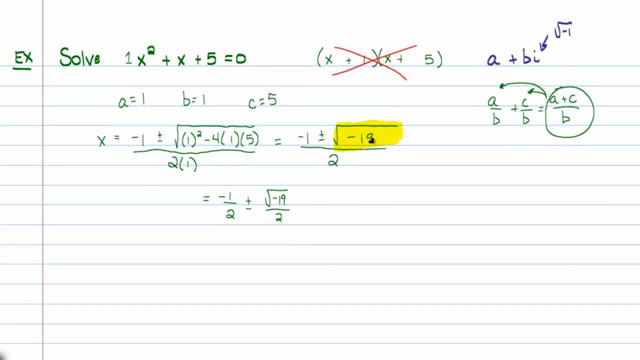 So in other words, it's negative 1 over 2 plus or minus the square root of negative 19 over 2. And now, we'll go ahead and write this as negative 1 half plus or minus... This could be written as the square root of 19 times the square root of a negative 1. All over 2. 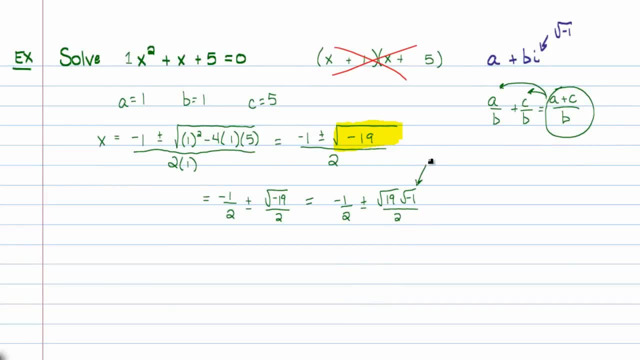 But now I know the square root of negative 1. That's just i. 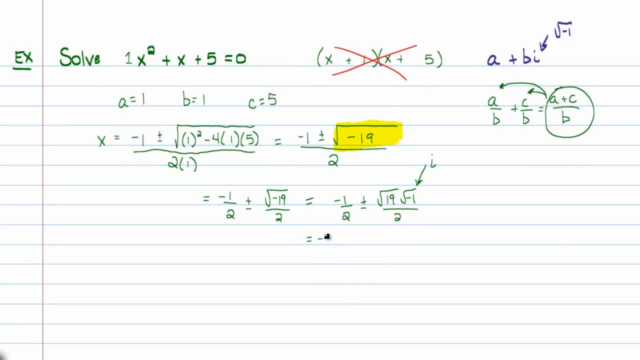 So this can be written finally as negative 1 half plus or minus root 19 over 2. And that's being multiplied by i. That is written in complex number format. 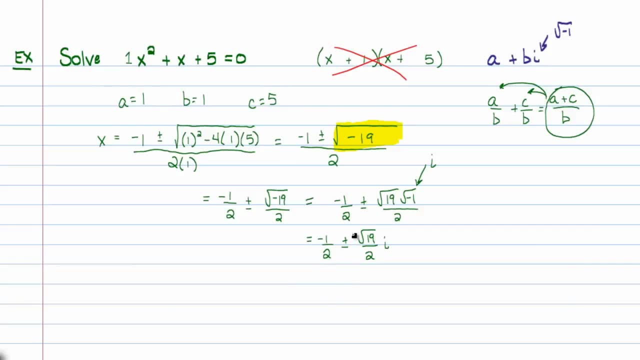 What's interesting about this... If you just look at the basic form. Ignore the fact that we have 1 halves and root 19 over 2's. It's in the form of number plus or minus some other number, i. Which is very interesting. 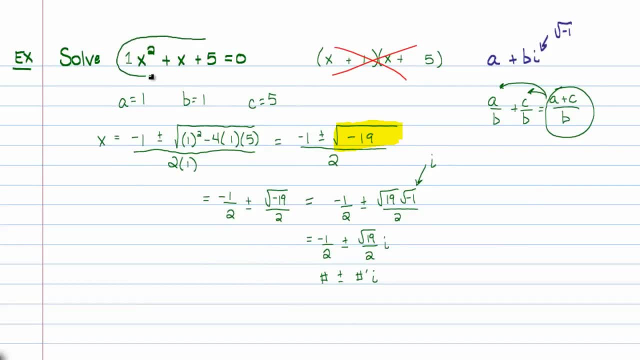 So I have a solution to this quadratic equation. And the solutions are negative 1 half plus some number i and negative 1 half minus that same number. Times i. 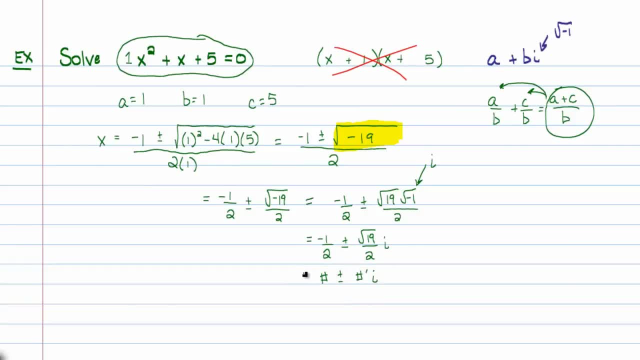 This plus or minus business introduces an idea called a conjugate. Now, often I will see it written in textbooks that authors will talk about this as complex conjugates. But I'm just going to call it a conjugate. The conjugate of the statement... A plus b i is a minus b i. 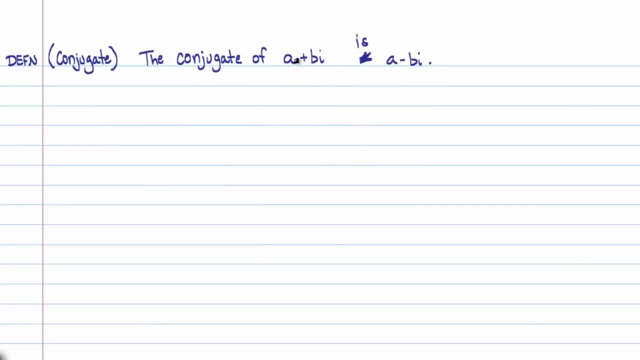 Really, all we're saying is that if you want to find the conjugate of a complex number. You flip the sign in the middle. 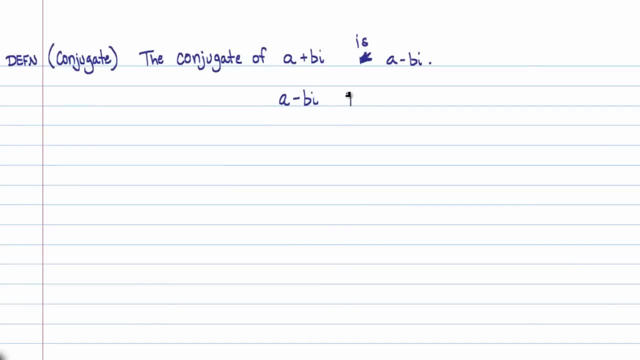 Same thing if you have a minus b i. The conjugate is a plus b i. So you're just flipping the sign in the middle. 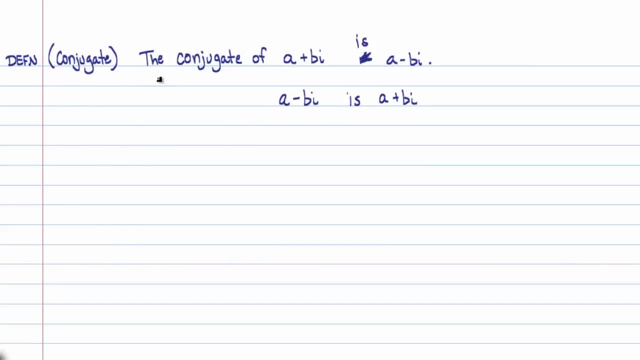 And what's interesting about conjugates is that... And not only just conjugates. But conjugates and solving quadratic equations. Is that when you solve a quadratic equation. 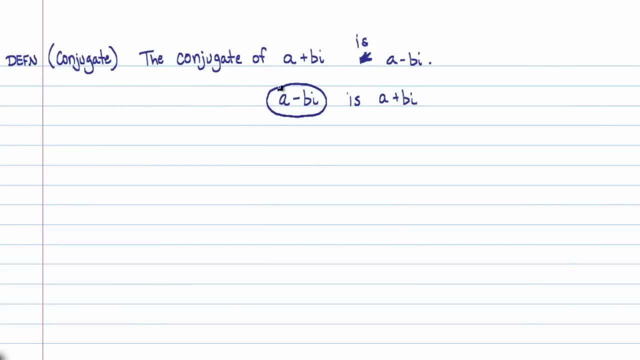 If you have a complex number solution. Like this. Then you also have its conjugate as a solution. And that's actually a theorem. So let me write that down. So if a plus b i is a solution to a quadratic equation. Then its conjugate a minus b i is also a solution. By the way this also holds. If a minus b i is a solution. 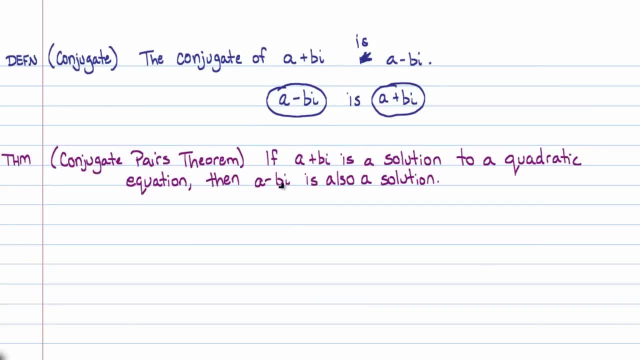 Then a plus b i is also a solution. Now I want to just state right now. That the point of this complex number conversation. Is not to get you to be an expert with complex numbers. Not at all in fact. All I want you to be able to do is recognize. A complex number solution to a quadratic equation. 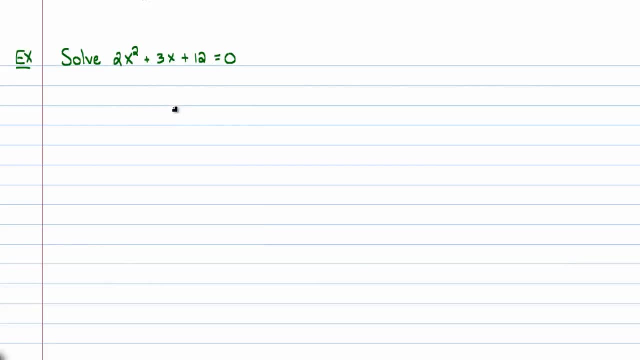 So let's go ahead and try to solve this quadratic equation right here. And see what happens. The first thing I'm going to do is see if I can factor this. 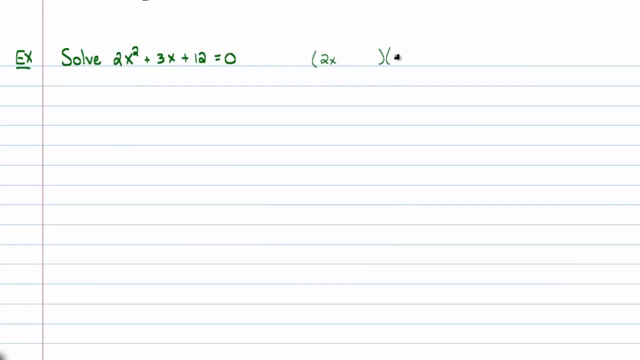 I immediately... You can already see it's not going to factor. 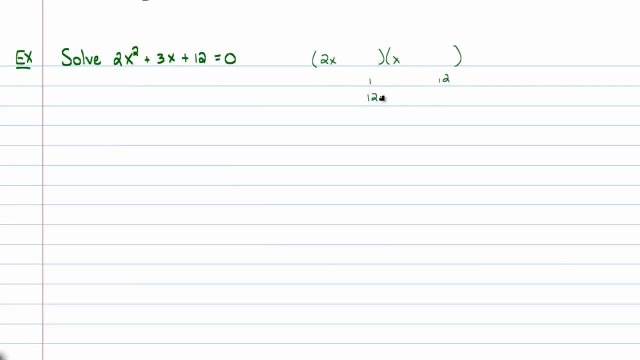 Two numbers that multiply to twelve is either one and twelve. Or twelve and one. Two and six. Or six and two. Three and four. Or four and three. 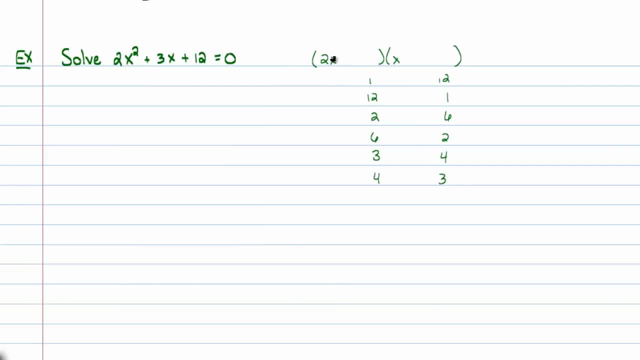 And if you check each of these. Try to make a combination of them to become three. Well I know two and twelve. Or I'm sorry. 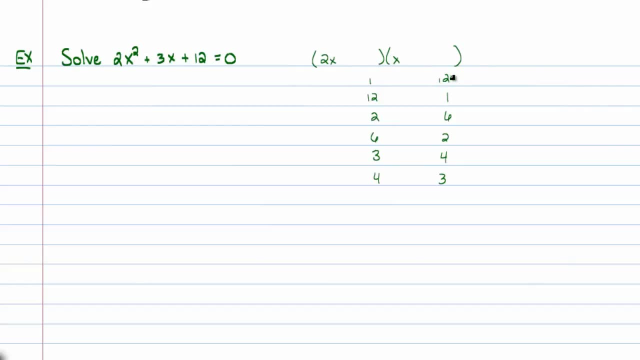 Two times twelve is twenty four. And one. Twenty four and one is... There's no possible way there. Two times one is two. 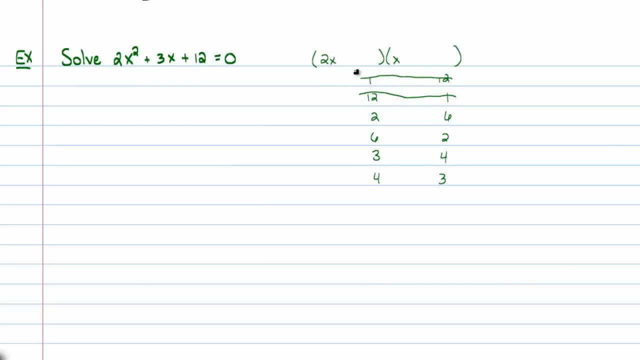 And then twelve times one is twelve. So two and twelve. No possibility there. Twelve and two. Again no possibility there. Four and six. No possibility there to get to three. Eight and three. No possibility. And six and four. 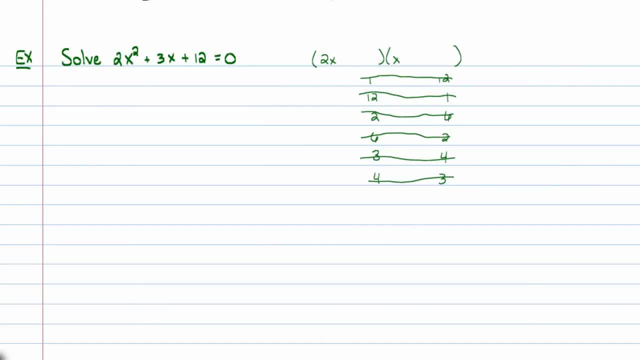 No possibility. So just kind of quickly checking through. There's no possibility to factor this. 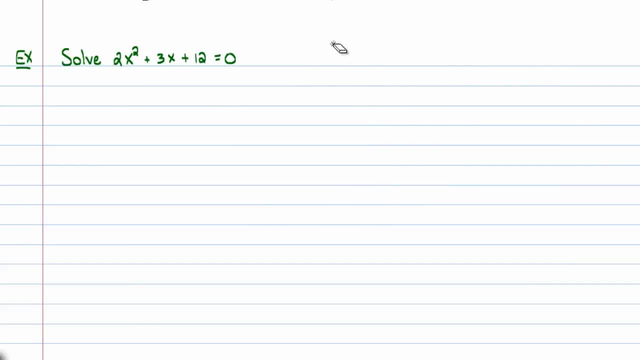 So I'll just erase all my tries. And now I know I'm going to immediately go for the quadratic formula. X is equal to the opposite of the B term. Plus or minus the square root of that B term being squared. Minus four times the A term. Times the C term. All over. 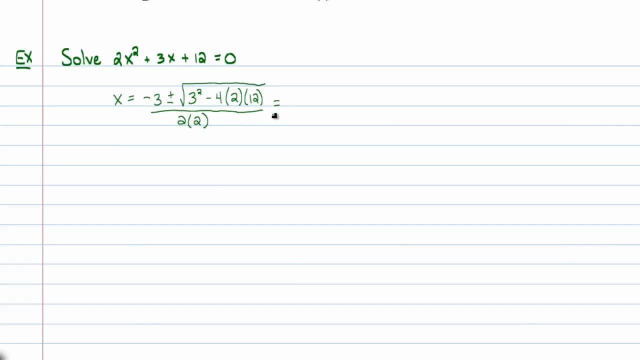 Two times the A term. Again I shouldn't be using the word terms here. It's the ABC. 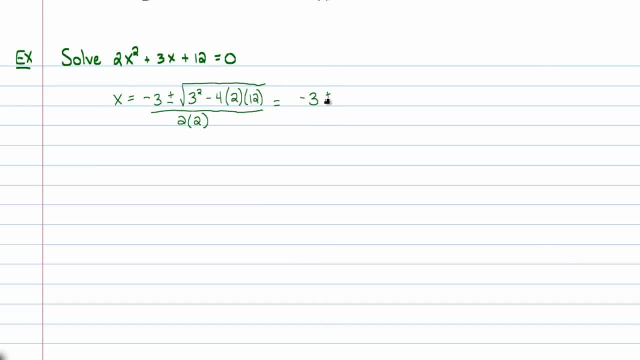 But I said it so I have to kind of stick with it. So that's negative three plus or minus the square root of. Let's see. I have twenty four times four. 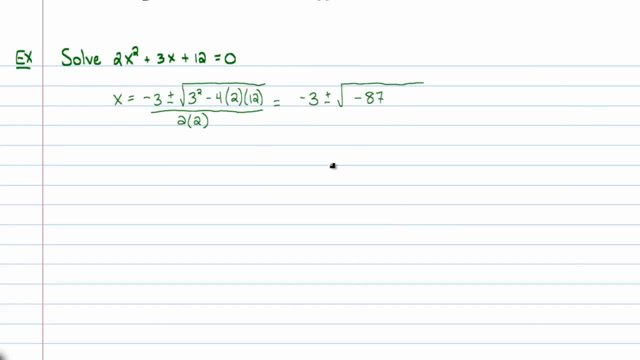 Which is a negative eighty seven. 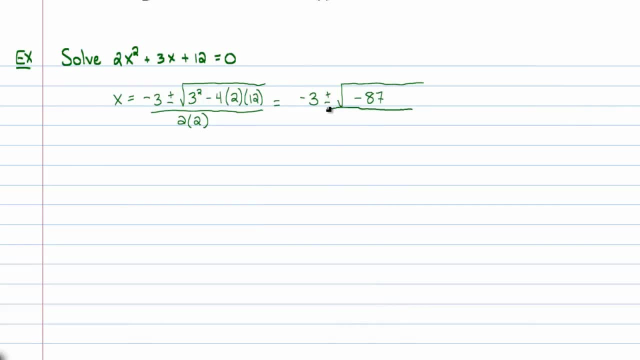 As I think about it. Yeah. All being divided by four. 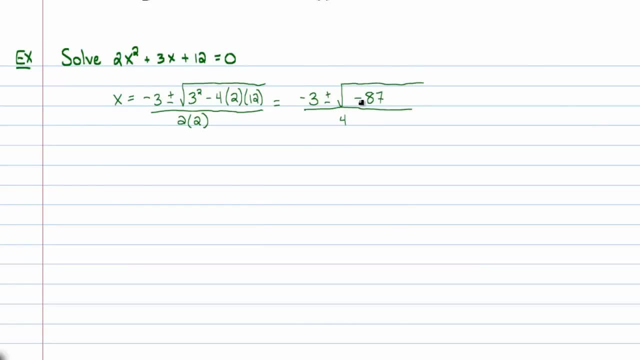 So at this point I need to really write this in terms of a complex number. So I will do this negative three plus or minus. I'll write this as the square root of eighty seven. 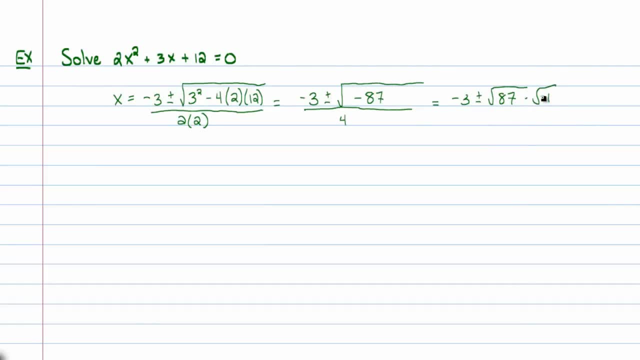 Times the square root of a negative one. As you can probably see. 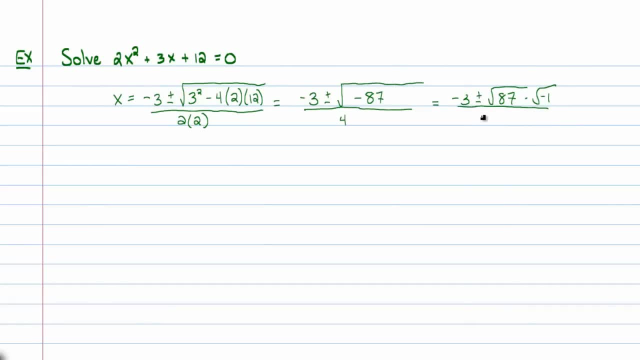 Negative one times eighty seven is going to be a negative eighty seven. So that is proper. 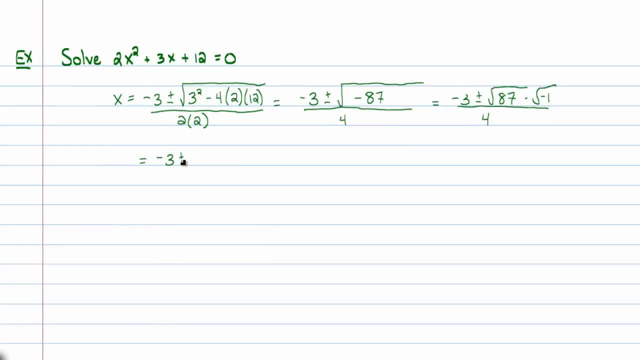 And. I could rewrite this as negative three plus or minus. 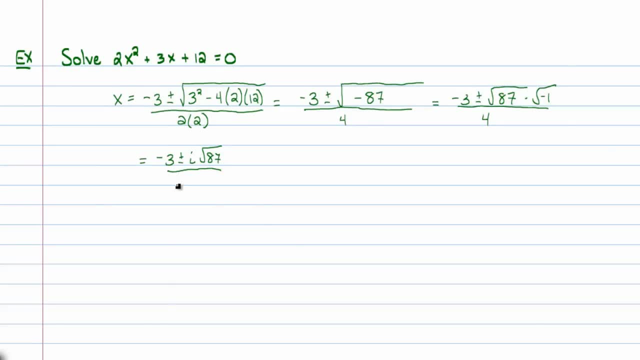 I times the square root of eighty seven. Now. What I want you to recognize here is that I'm writing the I. 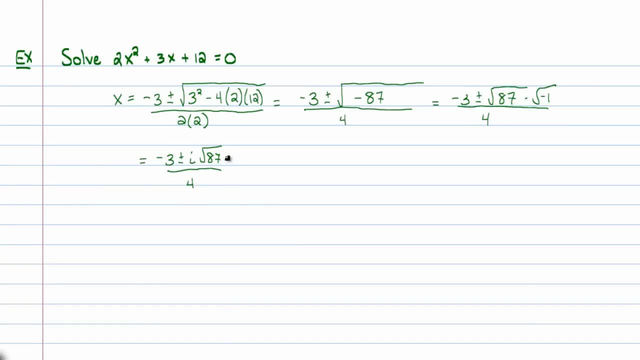 In front of the square root. The reason why is just a good habit to get into. Writing an I at the back end of the square root. Sometimes fools people into thinking that it's underneath the square root. And it's not. An I never goes underneath the square root. So that it just sticks out front. It's just easier. Better notation to leave it. Leave the variable out front. Even though it's not a variable. But leave the letter out front. 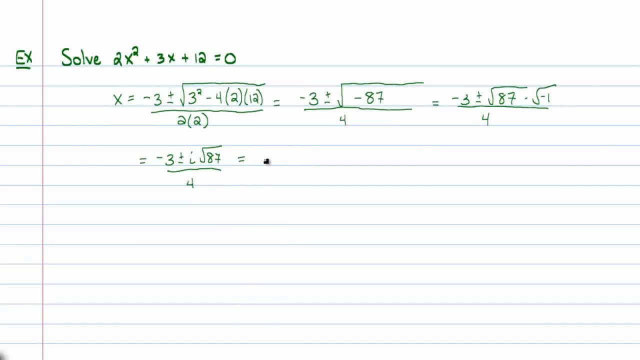 And now I'll write this in complex number form. That's a negative three fourths. Plus or minus. Root eighty seven over four. All being multiplied by I. And that's a complex number form. And notice that. 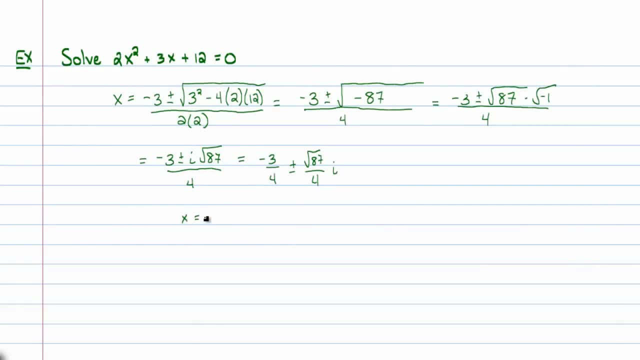 We actually do have. The solutions are conjugates. In other words. The solutions are a number. Plus. Root eighty seven fourths I. And. The other solution is actually it's conjugate. A number minus. Root eighty seven. Fourths. Times I. 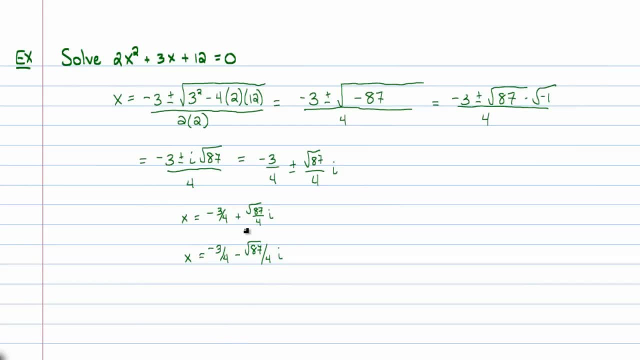 Very interesting result. But it's always that way with complex numbers. That. This. Solutions complex numbered solutions come in conjugate pairs. 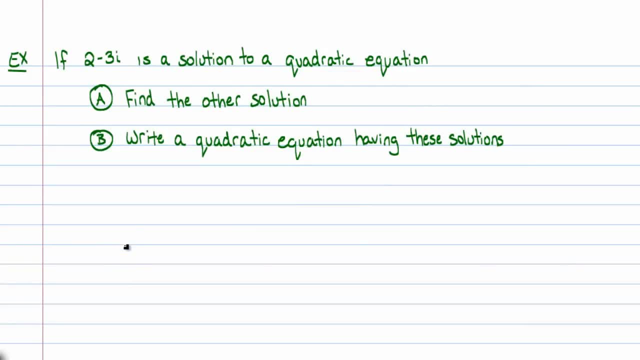 As a very. Advanced. Problem. 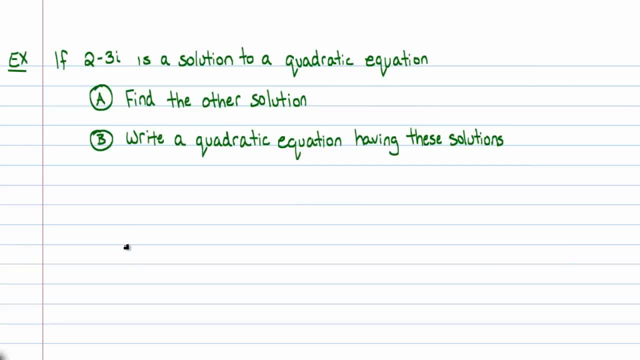 When you're dealing with. Complex. Numbered solutions for quadratic equations. You can consider this. Problem here. Let's suppose that we know a solution to a quadratic equation. 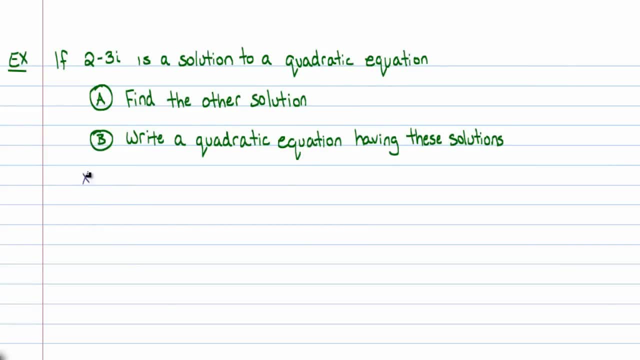 Is two minus three I. So we have a quadratic equation and we happen to know. That X equals two minus three I is one of the solutions. 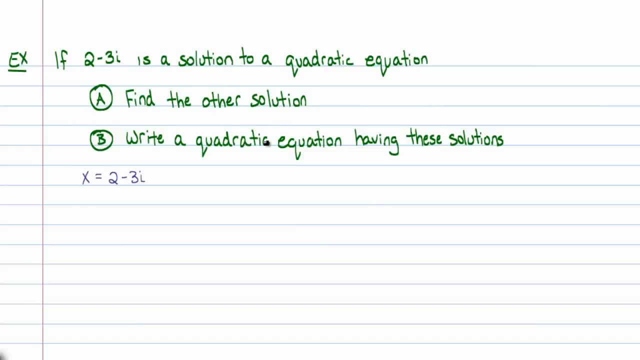 Can we find the other solution without. Any work basically. And the answer is yes. 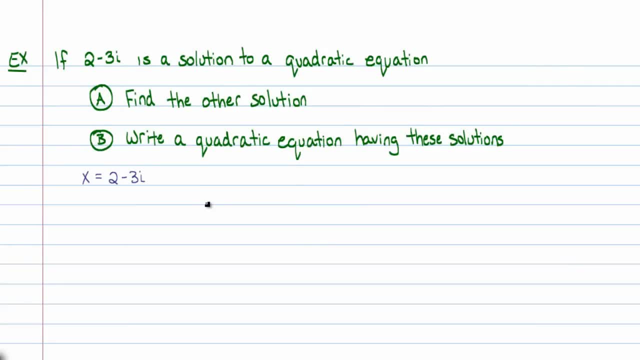 According to the. Conjugate. Pairs theorem. 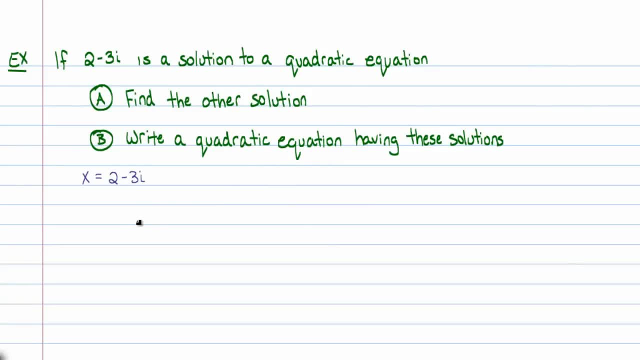 If two minus three I is a solution. Then it's conjugate. Two plus three I. Is also a solution. 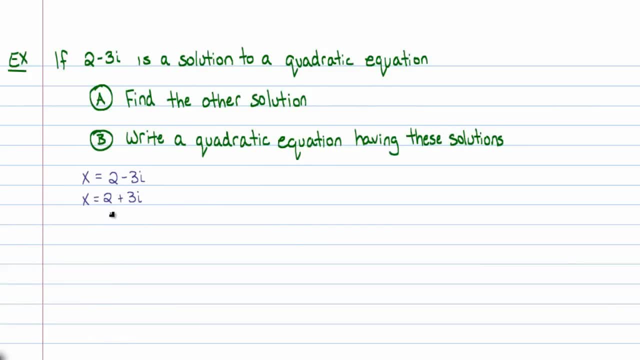 So these are our solutions. And now we want to write a quadratic equation having. These solutions. 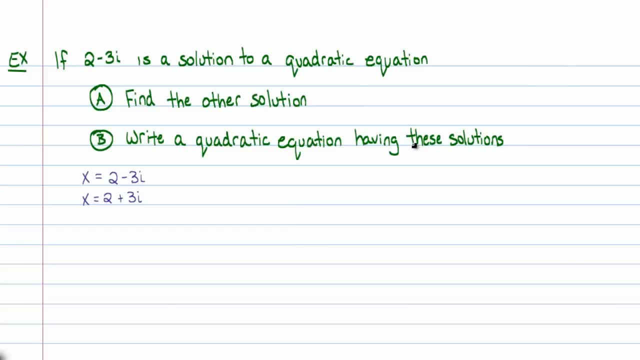 And now this is kind of the challenging part initially for students. I'll show you how it's done. 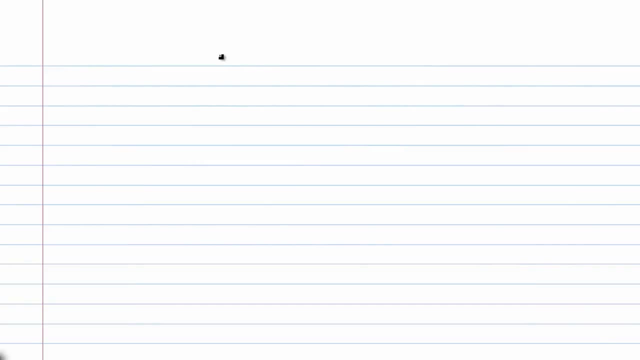 By taking. A side example here so let me hop over and just say well suppose we had. 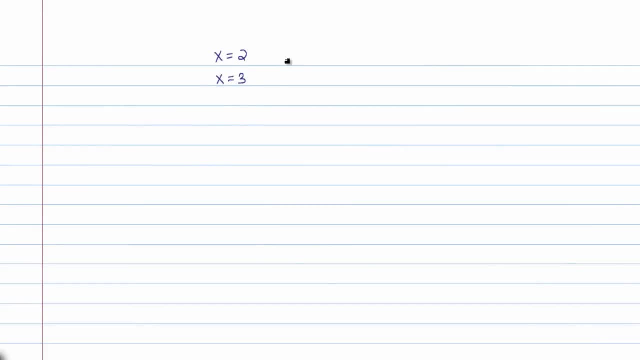 A quadratic equation that had these two solutions. Well. That would imply. That X minus two is equal to zero or. X minus three is equal to zero. Right because that's me subtracting two from both sides of this equation. And three from both sides of the second equation. 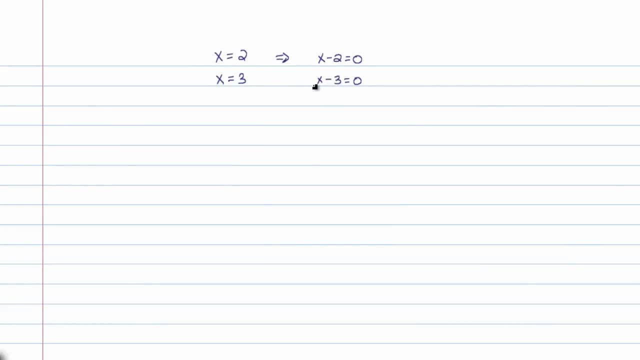 And now since. Either the first or the second object is equal to zero. 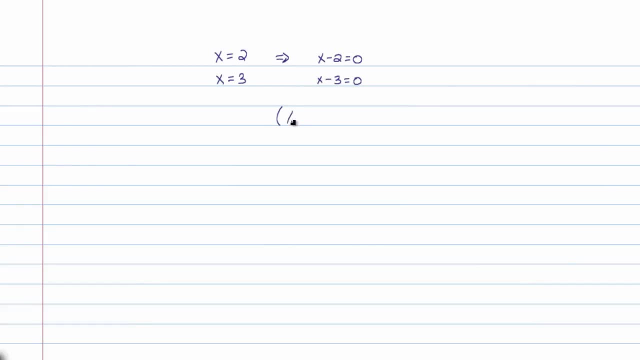 When you multiply these two things. Their product has to be zero. 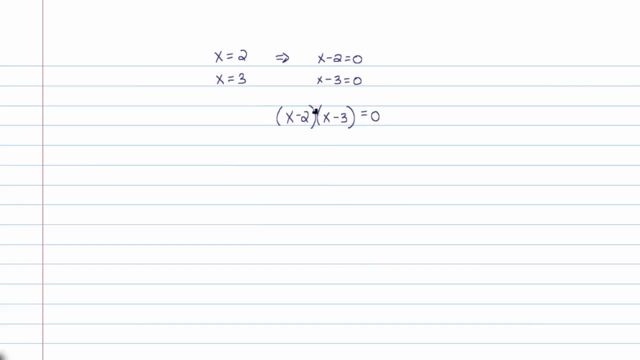 So when you multiply these two binomials. The product must be zero. And now you can see. 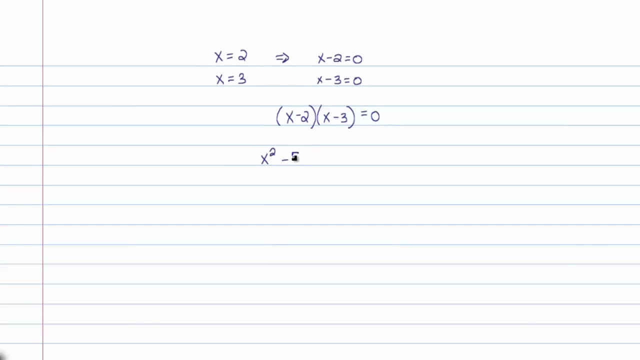 I could just distribute this out. I get X squared minus five X plus six. Is equal to zero. And that's the quadratic equation. Right there. 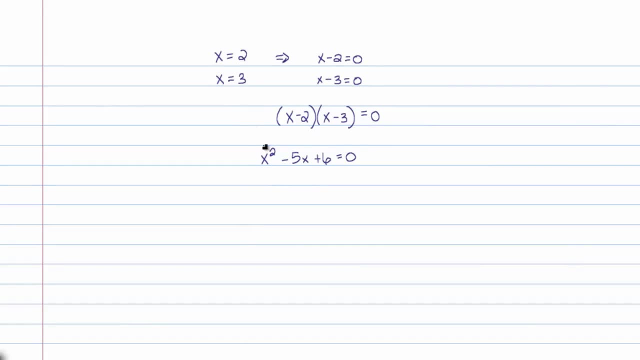 That has X equals two and X equals three as its solutions. 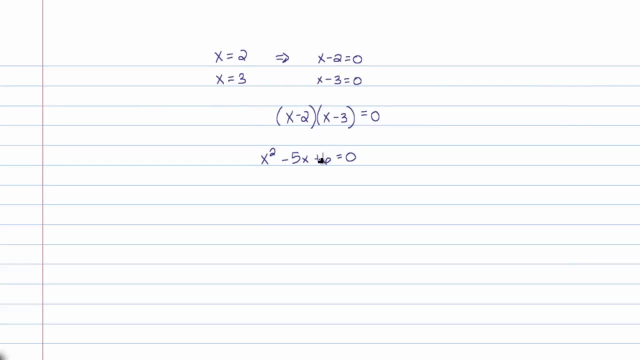 So we're essentially. Going backwards. Normally when we solve a quadratic. We try to factor it. And then we solve those factors. Right. 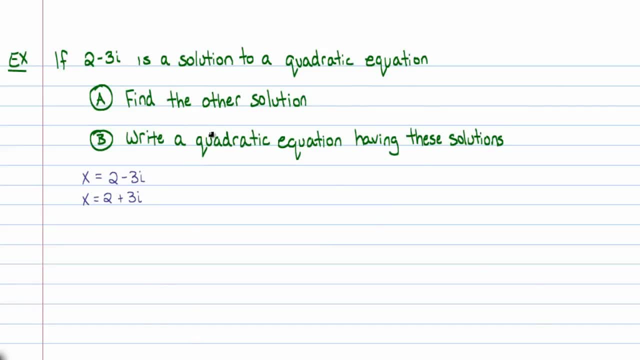 So. In the. Case that we're dealing with in this problem. 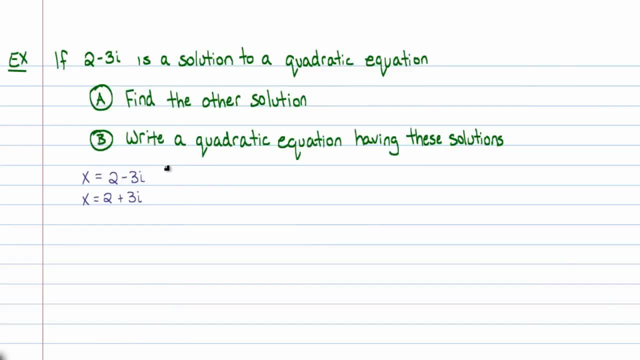 We're going to do the same thing. X equals two minus three I implies that. X minus two. Plus three I. Is equal to zero. 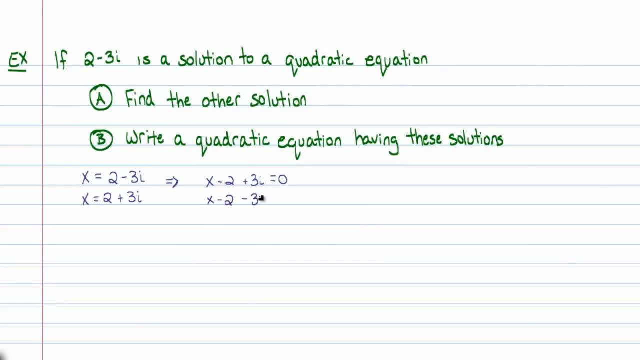 And X minus two. Minus three I. Is equal to zero. 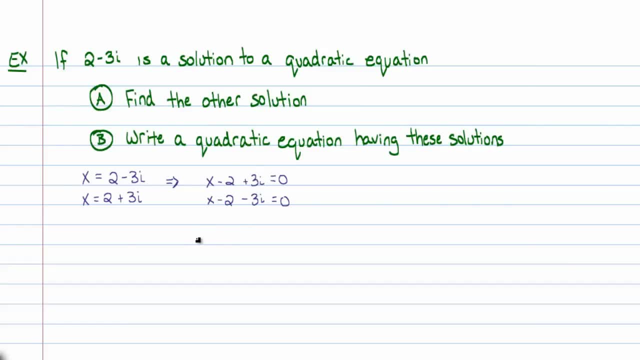 So if. Both of these statements are equal to zero. Then their product. Must be equal to zero. 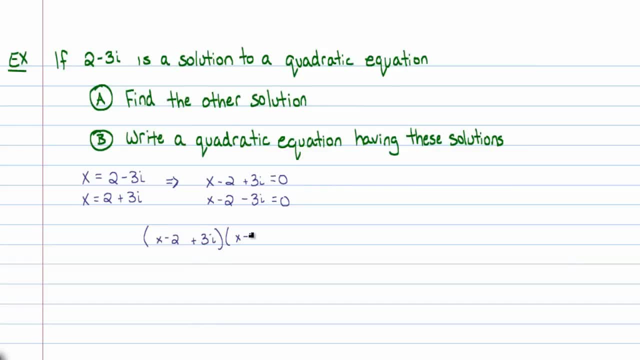 So. And now you can multiply this out. It's a couple ways you can multiply it out. You can either. Well there's a lot of ways actually. You can multiply this out. You can either stack it. 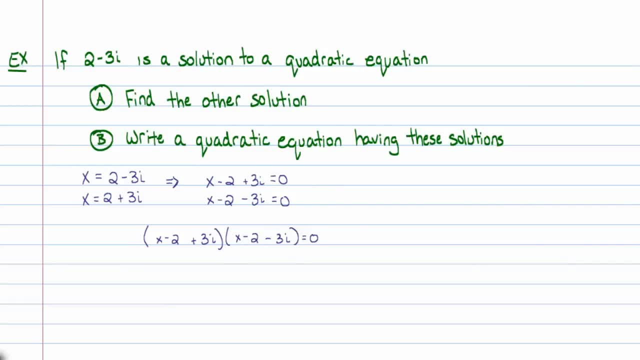 Or. You could distribute. I'll go ahead and distribute. Just to show how that this works. It's going to work just like regular distributions. 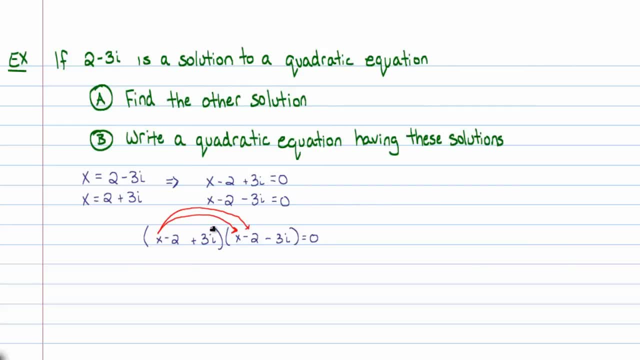 Don't be too intimidated. We'll have X times X. X times a negative two. And. Then. An X times a negative three I. And then. Do this in orange. 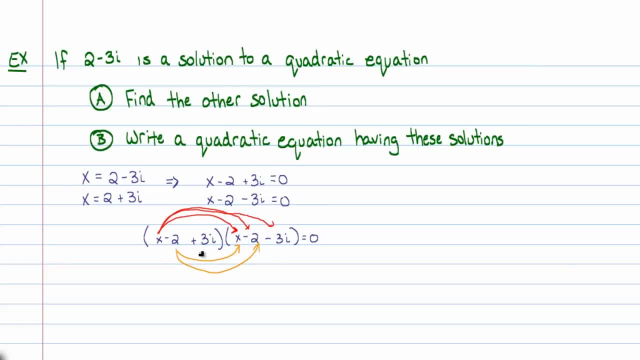 We'll have a negative two times X. A negative two times a negative two. 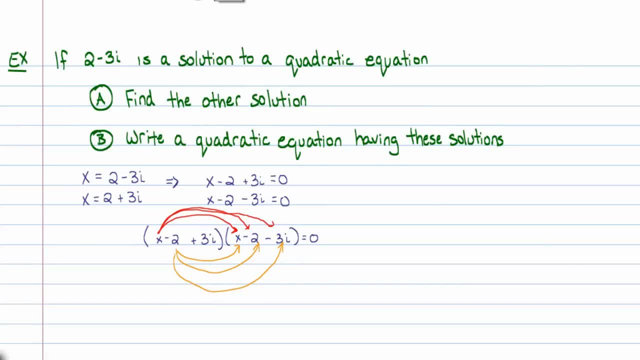 And a negative two times a negative three I. And finally. 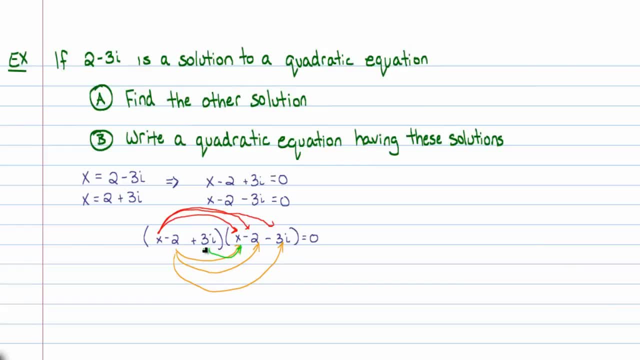 We'll have. I'll do this in bright green. Three I times X. Three I times a negative two. And three I. 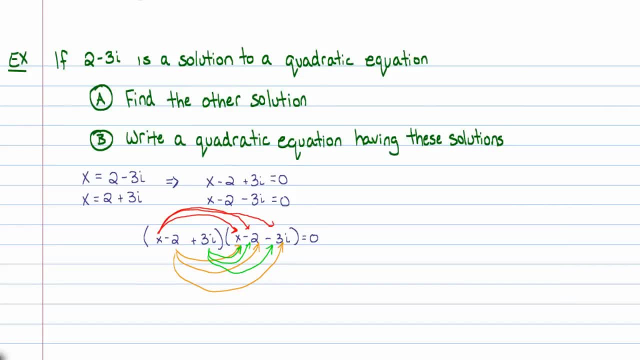 Is a negative three I. Here we go. 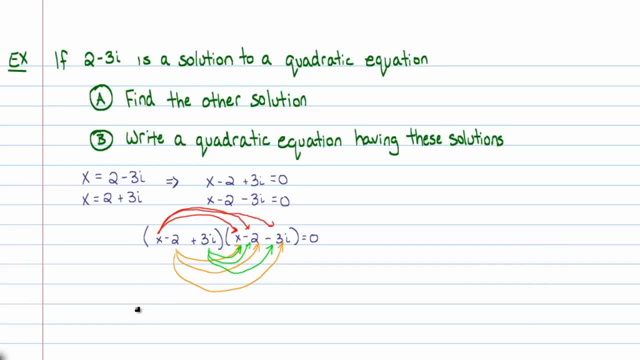 Let's go ahead and do this. We'll do the red stuff first. X times X gives me an X squared. X times a negative two. It gives me a negative two X. X times a negative three I. Is a negative three I times X. 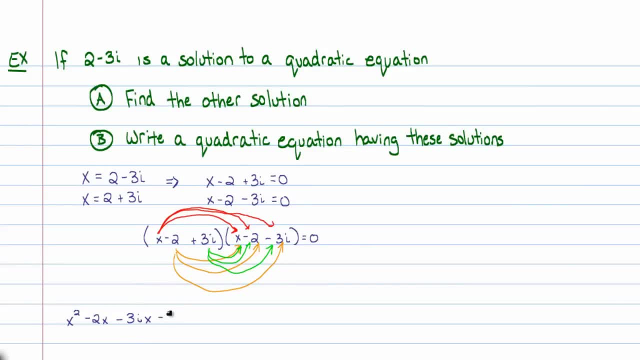 Now we'll do this stuff in orange. Negative two times X. Is another negative two X. And negative two. Times a negative two. Is a positive four. A negative two times a negative three I. Is a positive six I. And now we start going to the stuff with green. 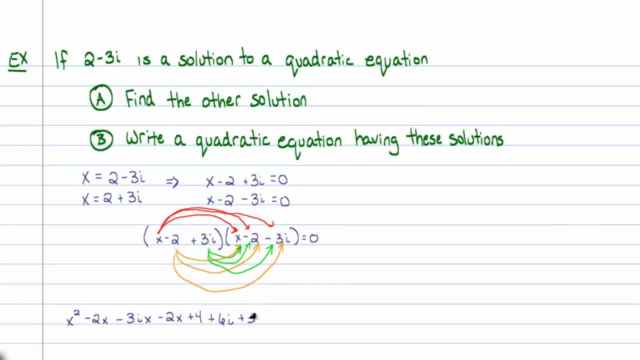 Three I times X. Is a positive three I X. 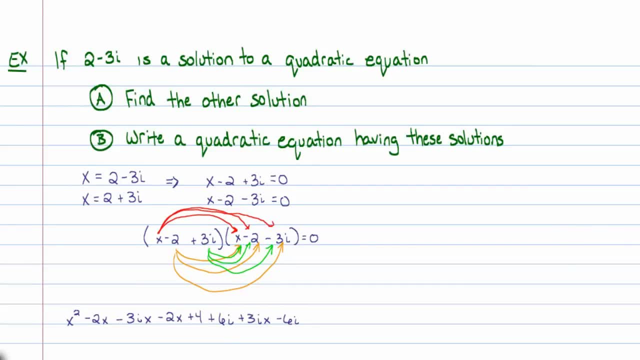 Three I times a negative two. Is a negative six I. 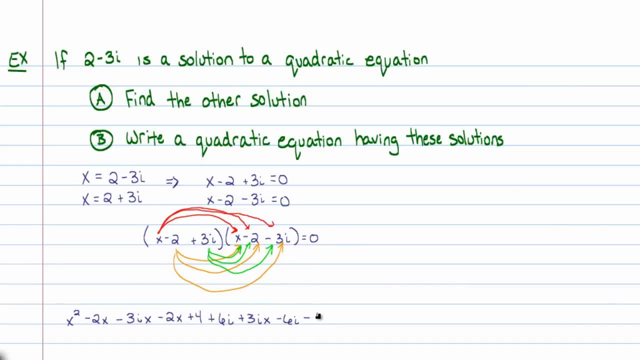 And finally. Positive three I times a negative three I. Is going to be a negative nine. I times I. Is an I squared. We'll talk about that in a moment. 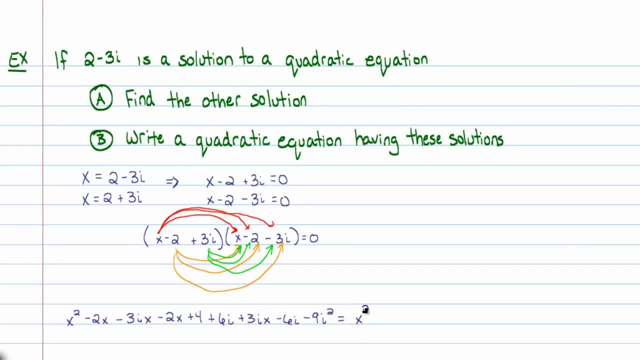 But let's at least combine like terms. I have an X squared. Let's see. I have a negative two X. Lose another two X. Gives me a negative four X. I have an. And let me cross out my. 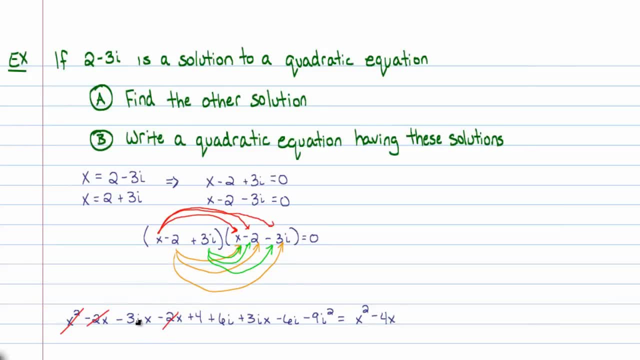 The stuff that I've worked on here. I have a negative three I X. But I'm adding back a three I X. So those two cancel. I have a positive six I. But I'm losing six I. So those two cancel. I have a plus four. So let me write that down. 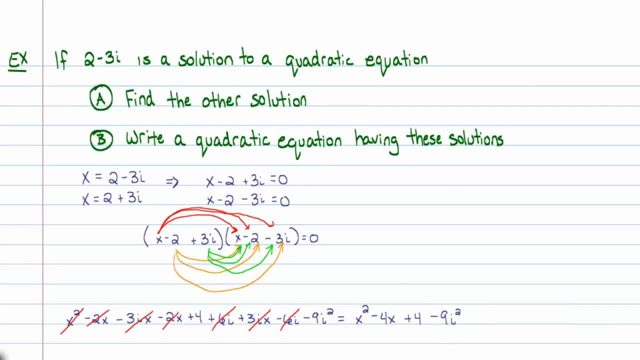 And then I finally have a minus nine I squared. Now there's something about the I squared that you should know. If I is defined to be the square root of a negative one. If we square both sides. I squared will be well. Negative one. It's the only number. That when you square it. It becomes a negative one. 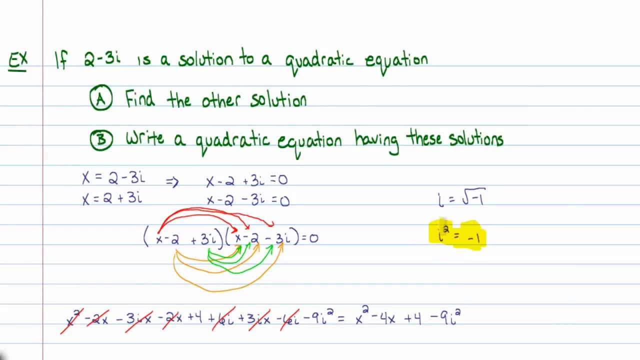 And that's a super important fact. 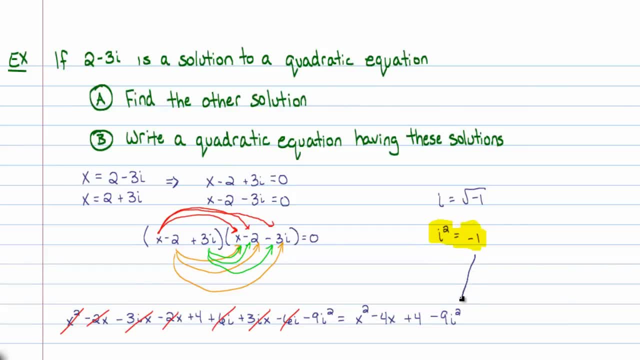 So what I'm going to do is replace. This I squared. With a negative one. So this will be. X squared minus four X. Plus four. Minus nine times a negative one. Or in other words plus nine. That's positive nine. Plus another four is thirteen. So the answer is going to be. X squared minus four X. Plus thirteen. 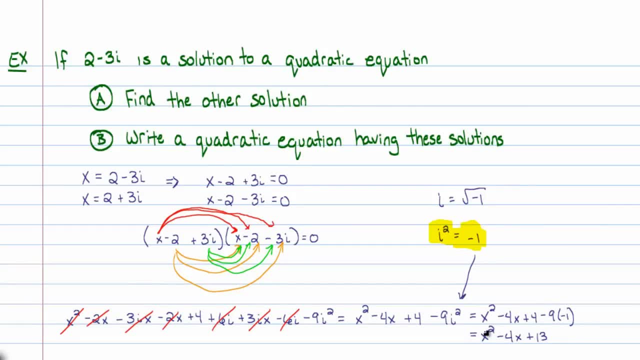 This is the quadratic equation. Well actually that's not. That's near to the quadratic equation. Having those solutions. 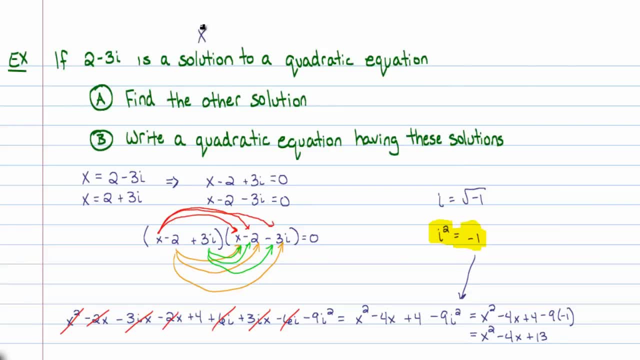 Technically. The quadratic equation having those solutions. Is going to be X squared. Minus four X. Plus thirteen. Is equal to zero. 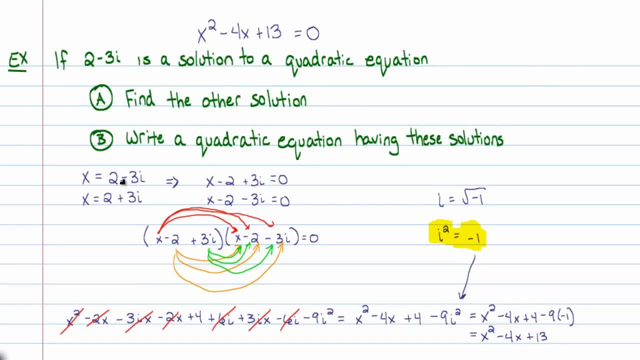 The solution to this quadratic equation. Is going to be X. Is going to be two minus three I. And two plus three I. A lot of work to that. But well worth it. You get a nice looking. Quadratic equation in the end. Very nice tactic. 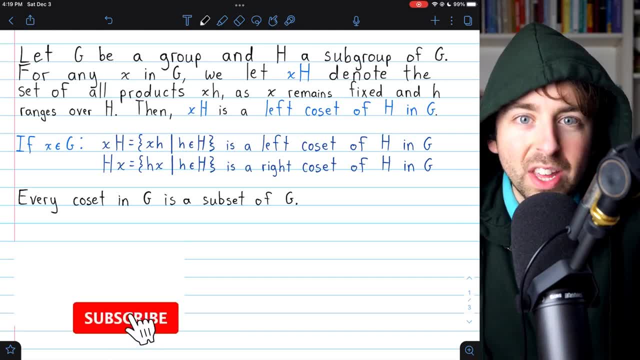 Today we're going to learn all about cosets in group theory and I think you'll be quite surprised by the importance of this definition and the results that all of this is going to lead to. 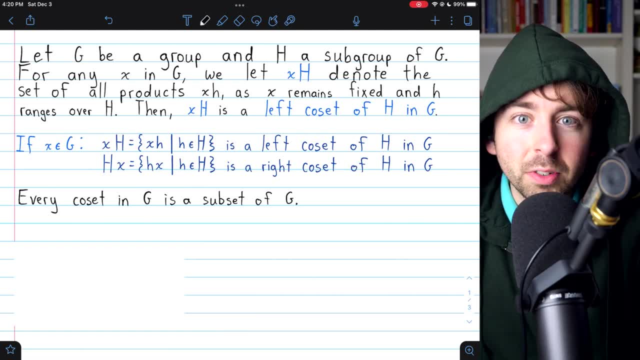 Not long after this we will attain a full understanding of every group with a prime number of elements. So this is some really cool stuff. In this video we'll go over the definition of coset. We'll see some examples both finite and infinite and we will cover a couple of the important results concerning cosets and we will do a simple proof proving that if two cosets have common elements they must in fact be the same cosets. Let's get into it.